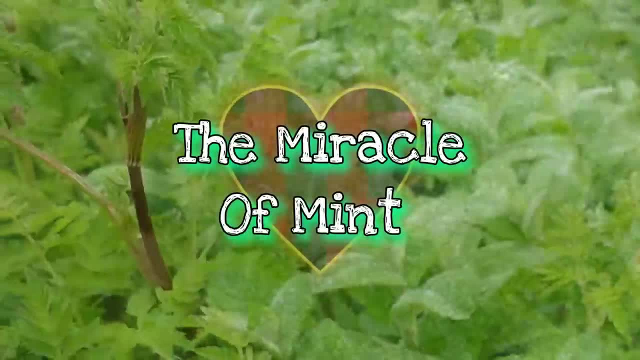 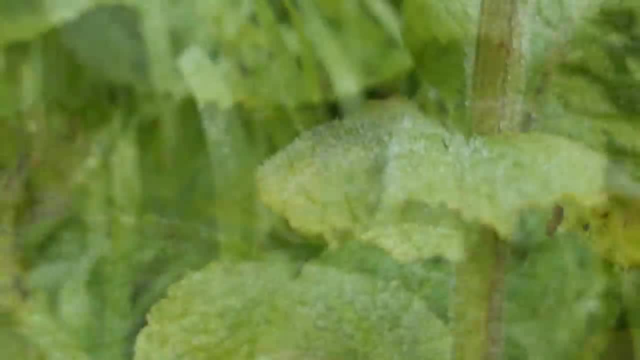 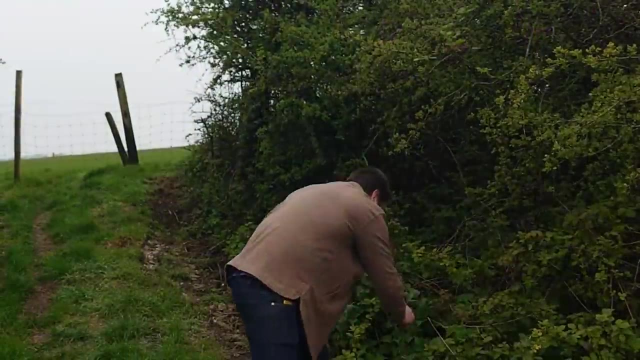 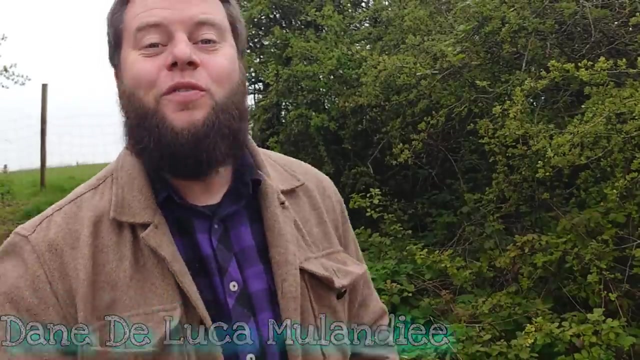 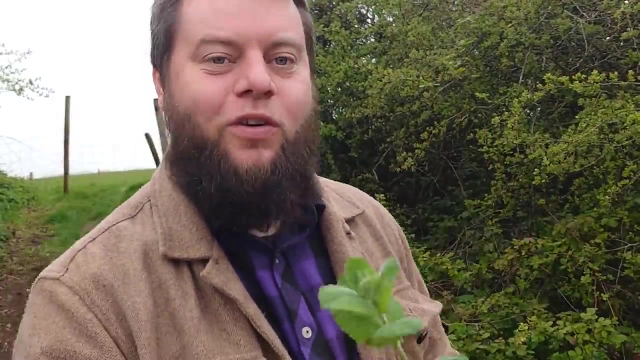 Hello, my friends, and welcome back to our channel. Home is where our heart is. My name is Dane, author of the series of books Knowledge to Forage. I hope you're having a beautiful day wherever you are in the world, and thank you all for joining me here on this beautiful spring. 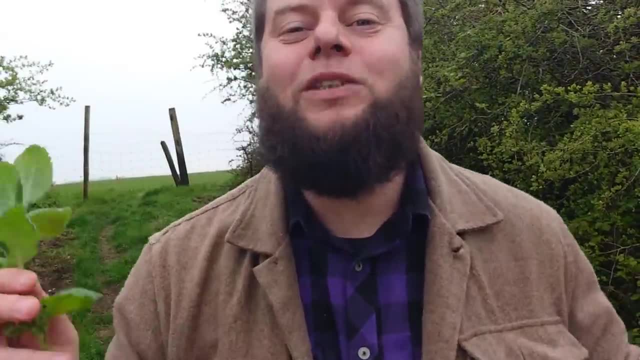 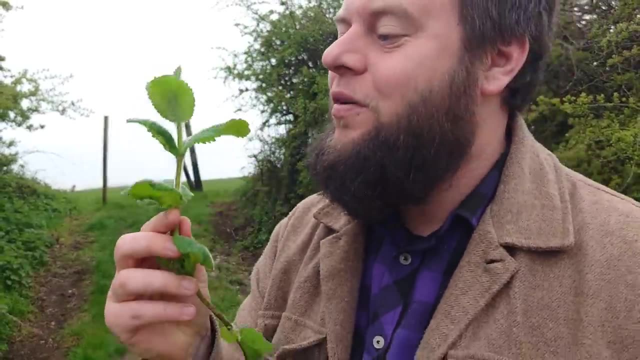 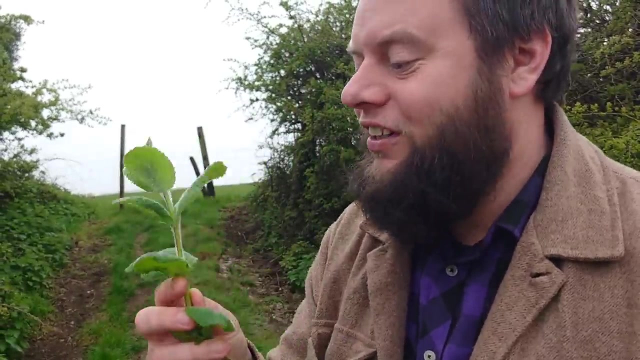 morning Spring has sprung and today a very special plant has caught my eye, and this plant is the wild mint. The mint is probably one of the most famous plants in the world today. It's used for teas, ice creams, chocolates. It gives bubble gum that refreshing, cooling feeling when we breathe. 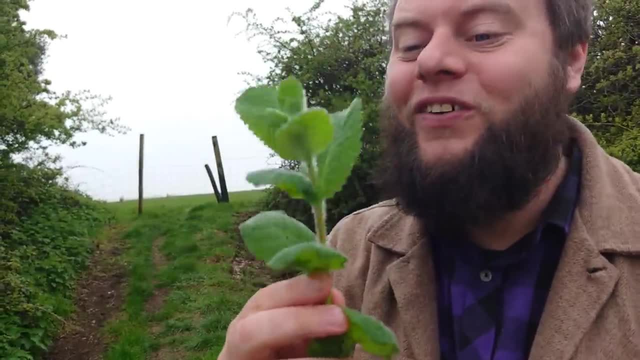 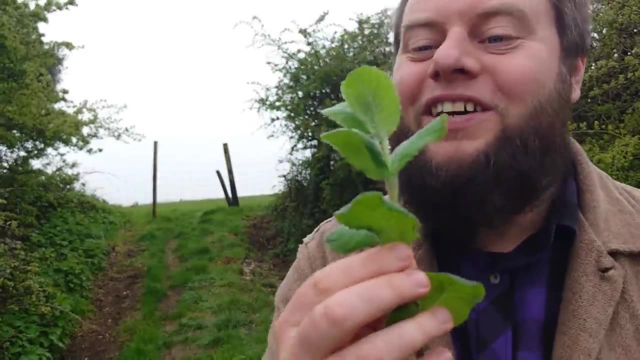 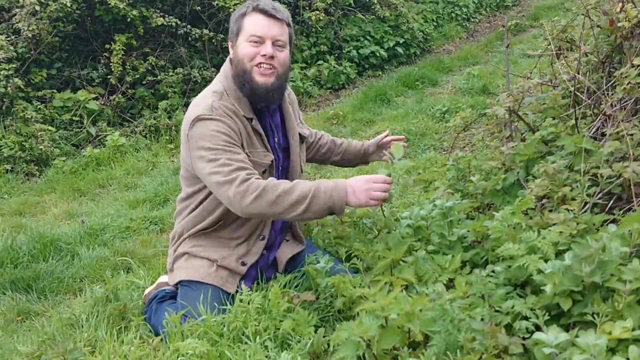 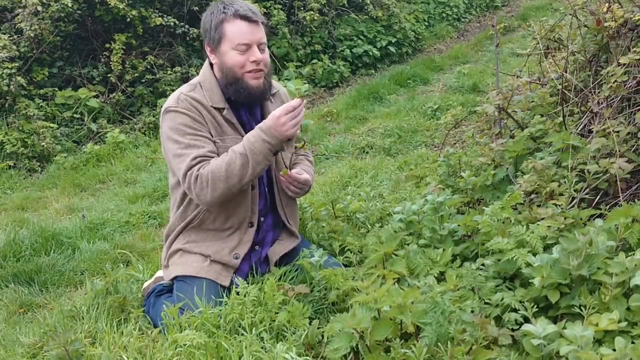 it out, and it's also a powerful medicinal plant too. So if you're interested, then come for a walk through the countryside with me and let's dive into the wonderful world of the mint. So here we have a giant patch of wild mint. Mint's incredible When we squish its leaves in our fingers and breathe in the minty essential. 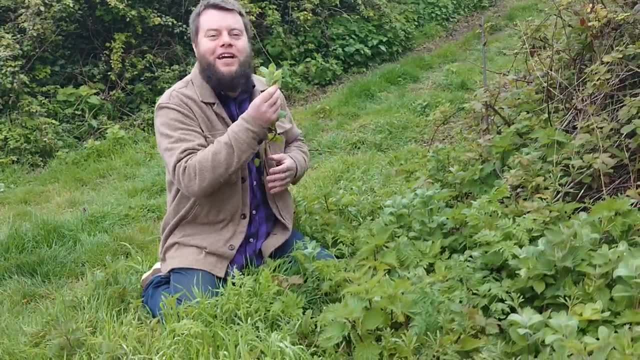 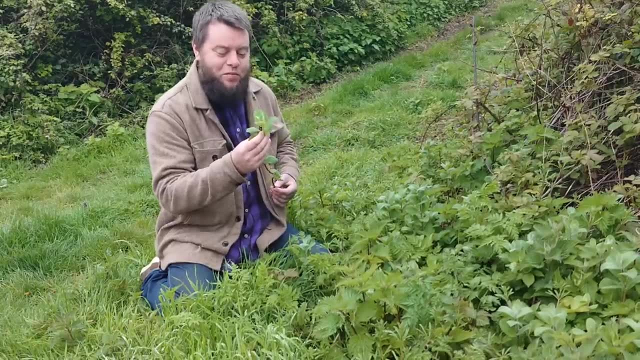 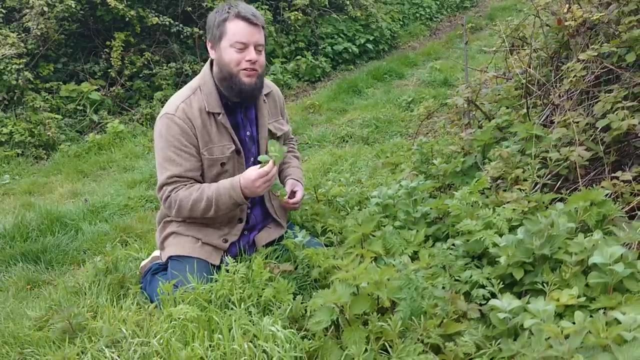 같. There's nothing there to silence itself. It washes away all our faults and it just leaves us and the mint. Now, what's awesome about mint is there's actually more than 600 types of mint that grace this good world. When you're out on your travels in the wild, you'll most likely come. 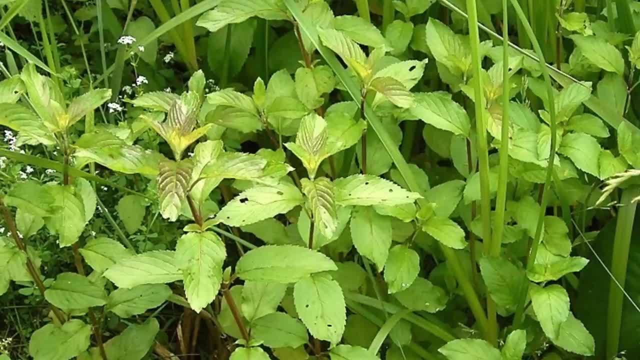 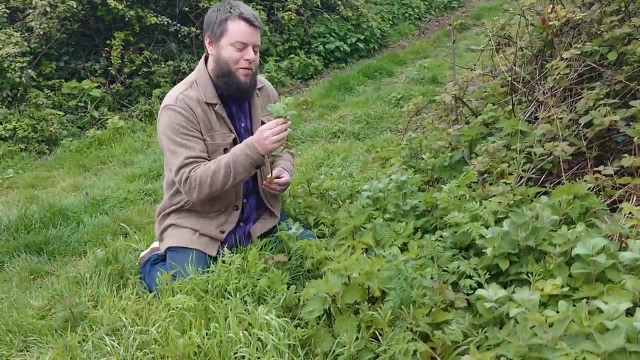 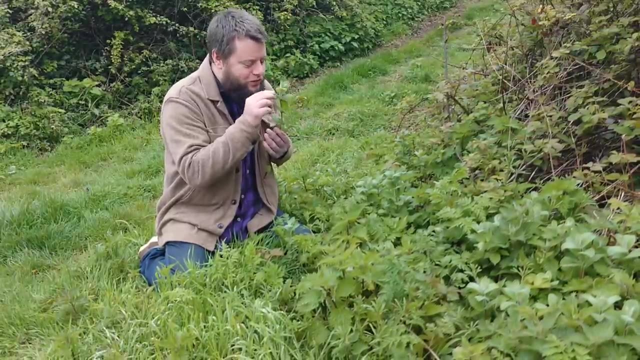 across peppermint, spearmint, water mint or, my personal favourite, what we have here, apple mint. Now, I absolutely love apple mint, also known as pineapple mint, because it's soft and fuzzy to the touch and it's essential oils. 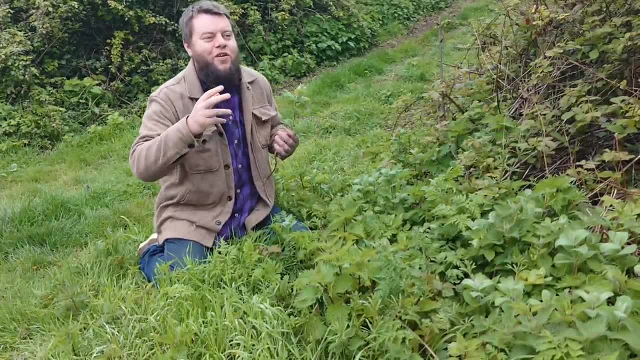 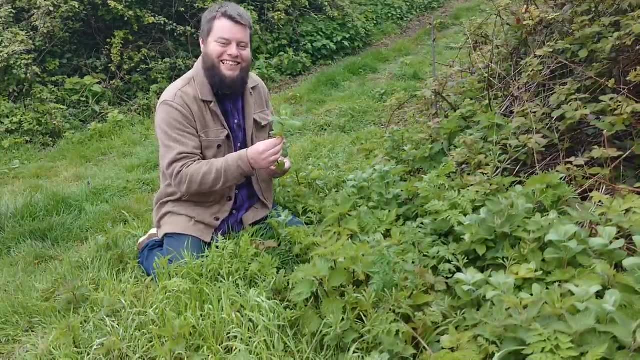 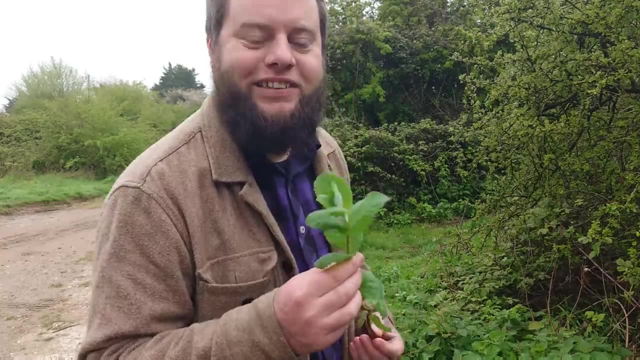 When you breathe them in, they smell like a mixture of warm mint, warm apples and warm pineapples, all mixed together in a bowl, And I love it. So when it comes to identifying mint, it's pretty simple. There's a lot of species of mint, but they all look pretty similar. 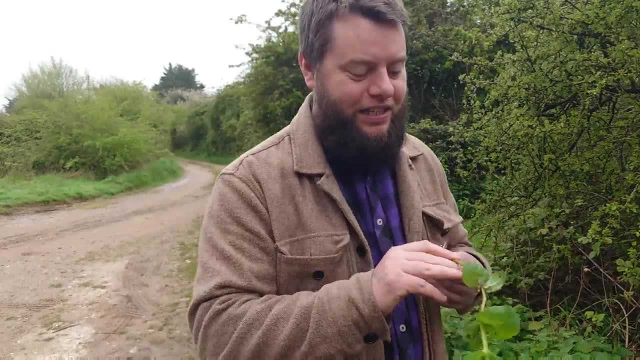 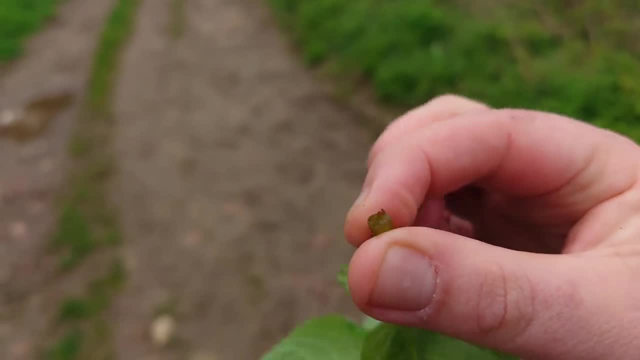 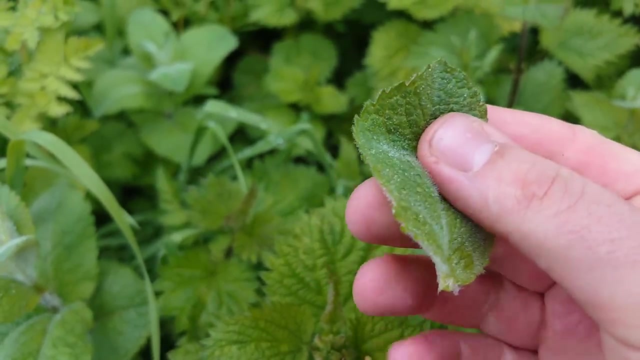 Firstly, all mints have a square stem. You see, when I roll the stem in my fingers, it's clearly a square. It's quite fascinating how things like squares can grow in love and nature. And for the apple mint, its leaves are quite rounded with lightly serrated edges, and the entire plant is fuzzy. 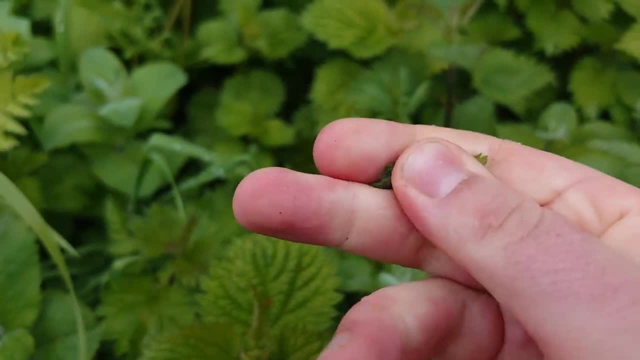 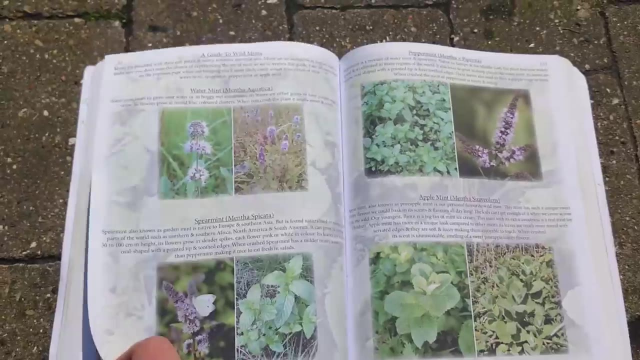 And when you crush the leaves it has that unique apple-y, pineapple-y, mint-y smell. Now in our book we've got an in-depth guide to mint, because we love it so much We don't want anyone to miss out on the blessing of mint. 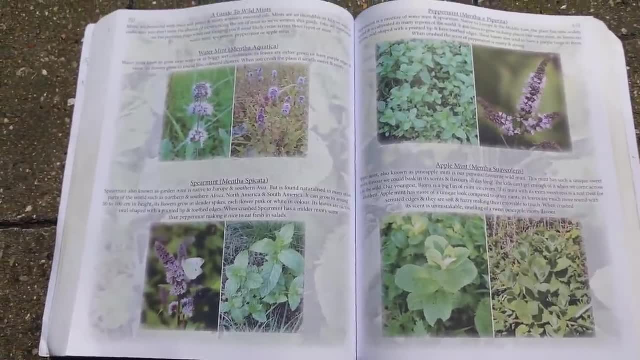 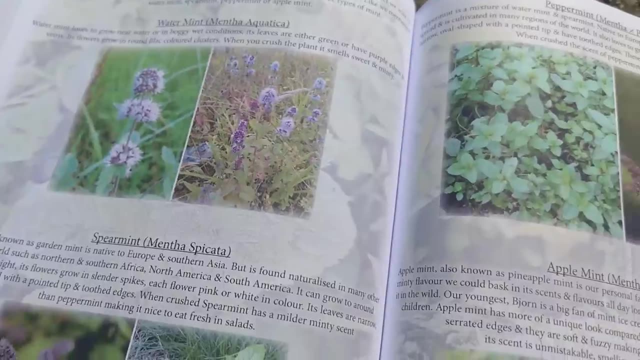 Check out our book for that in-depth guide on mint. And later on in the year, when mint plants grow up, they develop purple-y lilac flowers, and these grow in either round little spheres up the stem or like long cones off the top. 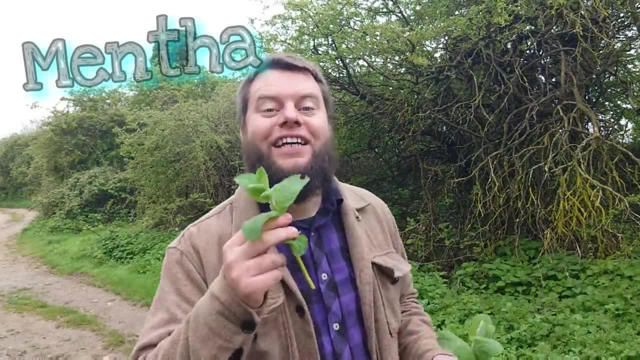 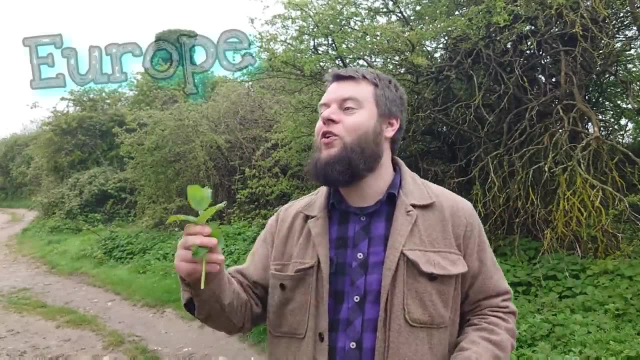 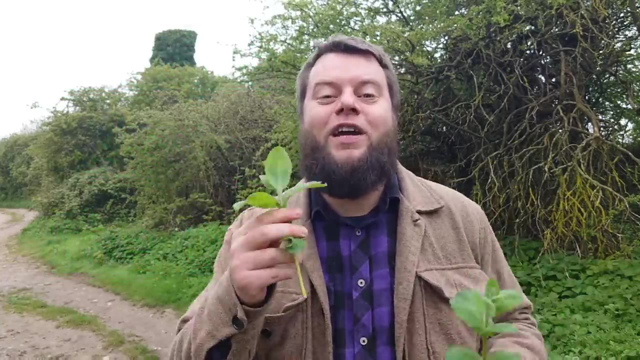 Now, mints are in the mentha genus, and they grow in abundance pretty much all around the world. You'll find them growing across Europe, Asia, North America, South America, Australia, And what's great about mints is they grow in abundance too. 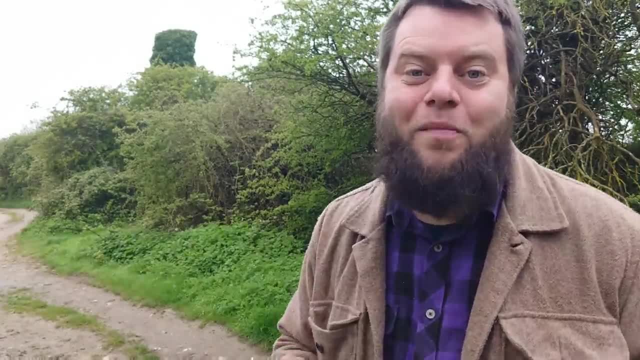 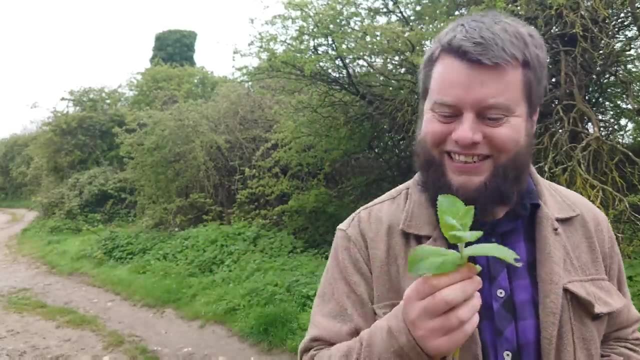 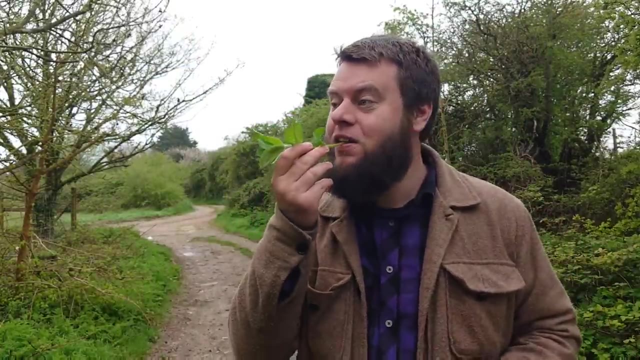 If you plant a single mint plant in your garden, for example, this plant will quickly spread and provide your entire family with all the mint it needs throughout the year. Now, when it comes to wild food, the mint is very special. You can eat it fresh and it has a very special cooling minty flavour. 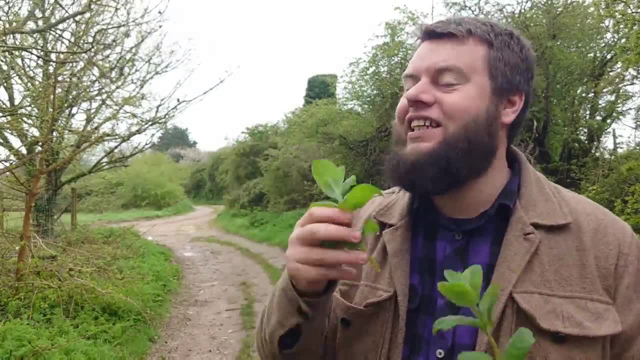 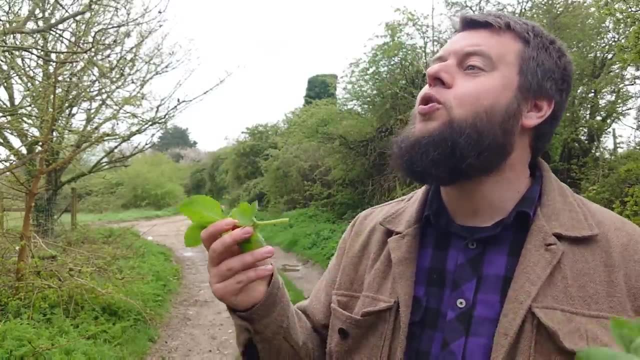 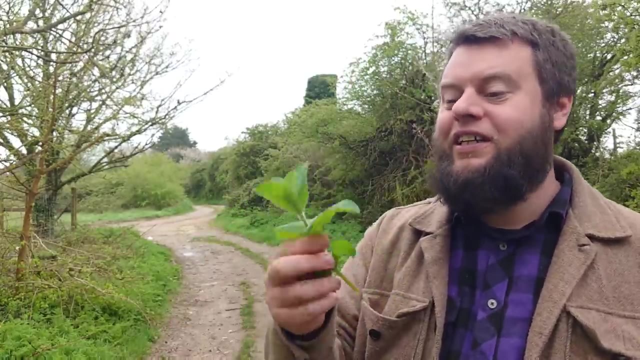 There's two great joys that comes with eating mint. Firstly, you get to eat it and enjoy this plant as a food source, a delicious minty food, And secondly, you get the joy of breathing out them powerful essential oils. Now the mint is commonly used dried into tea, and it's blended into ice creams, added to salads- you name it. 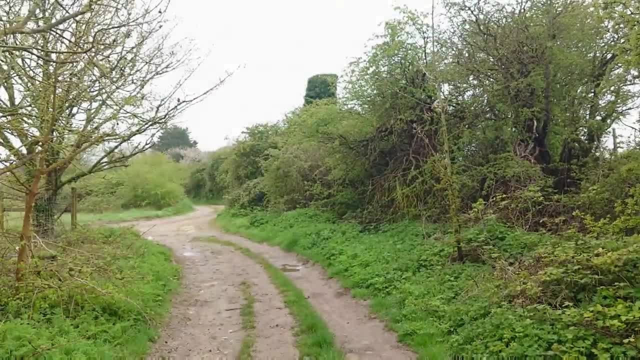 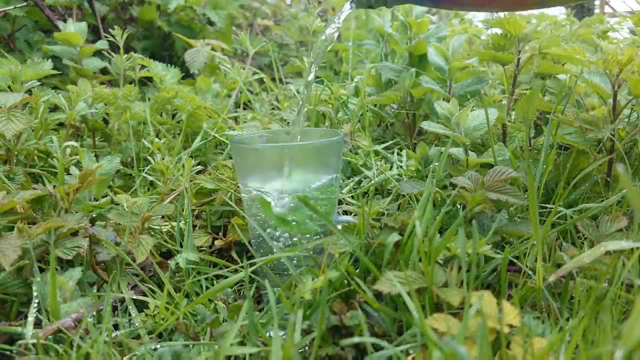 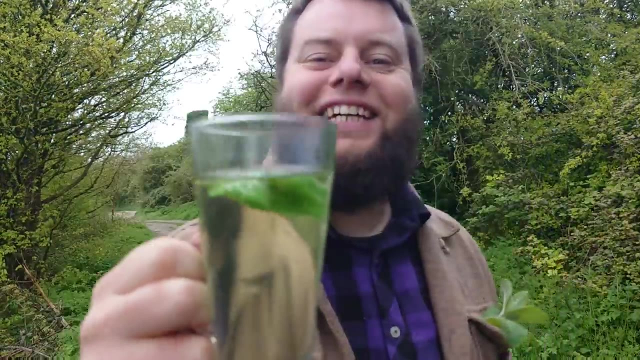 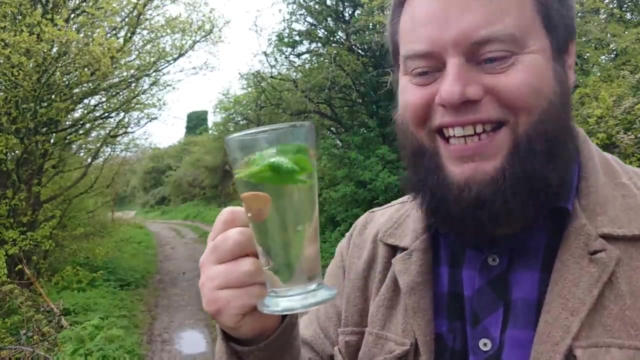 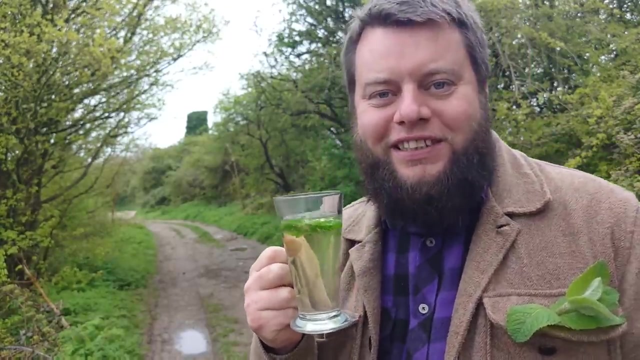 And the mint is used to flavour it. Ah, cheers, A refreshing cup of fresh mint tea. You don't get a better herbal tea than that. Now, what is giving mint this very unique scent and flavour? Where is this special refreshingness coming from? 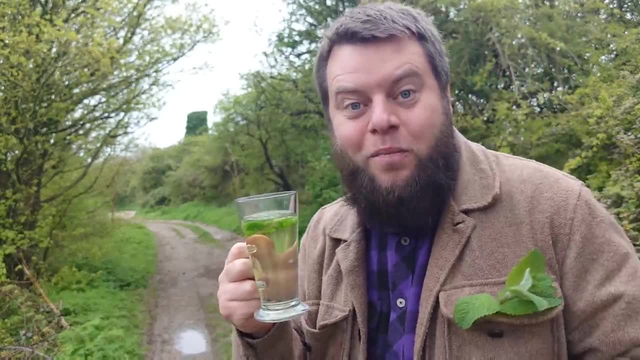 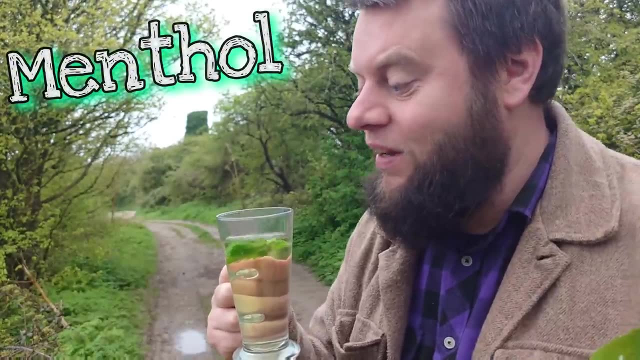 Well, what's actually happening here is, within the mint plant, a little miracle is happening and the plants creating an essential oil known as menthol. Now, it's this menthol that gives the plant this incredible refreshing scent, And it's also this menthol. 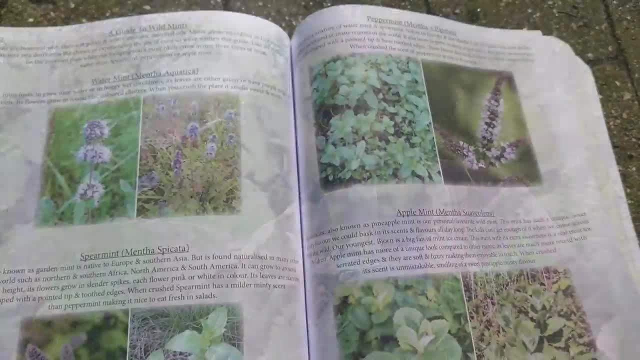 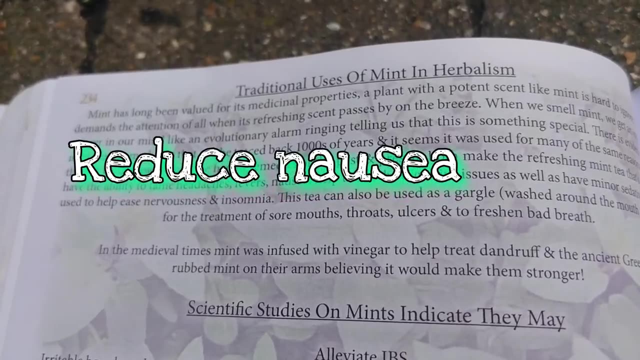 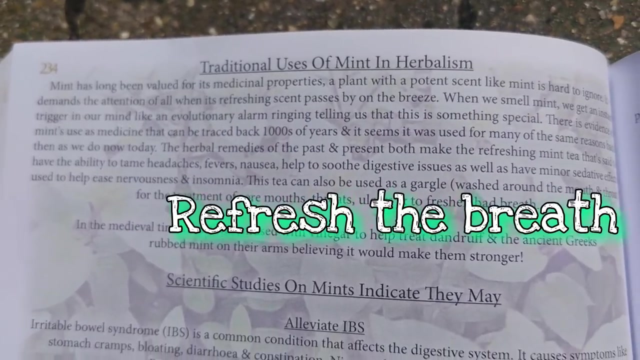 that gives the mint plant some of its medicinal properties too. In traditional herbalism, which is the knowledge passed down through the generations, mint was used as a tea to help us feel less nauseous when sick, soothe our headaches and digestive issues, as well as, of course, to freshen the breath. Mint would 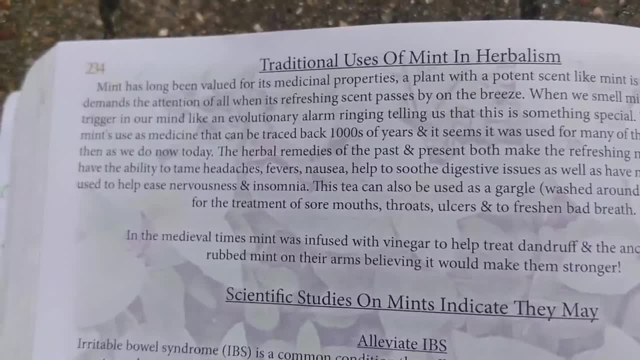 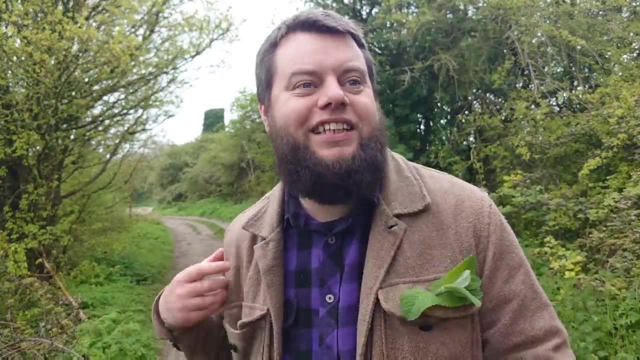 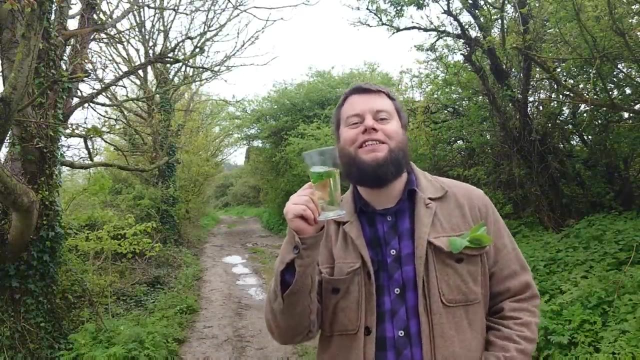 also be added to warm baths or packed into pillows to make herbal pillows. in times we'd feel really unwell, And the ancient Greeks would take the mint leaves and rub them into their muscles in the belief this would make them stronger. Mint's been a famous medicinal herb for thousands of years, and it was this that 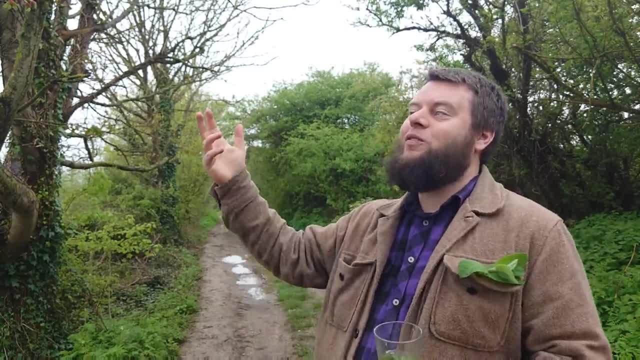 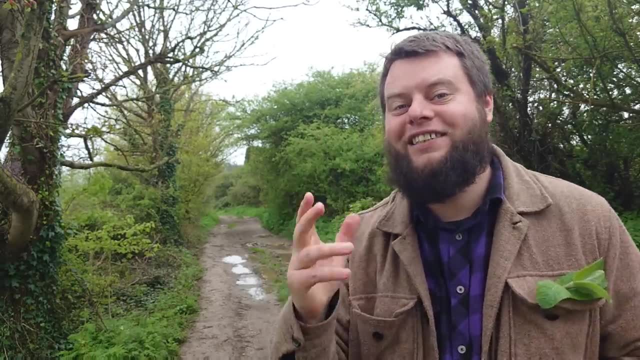 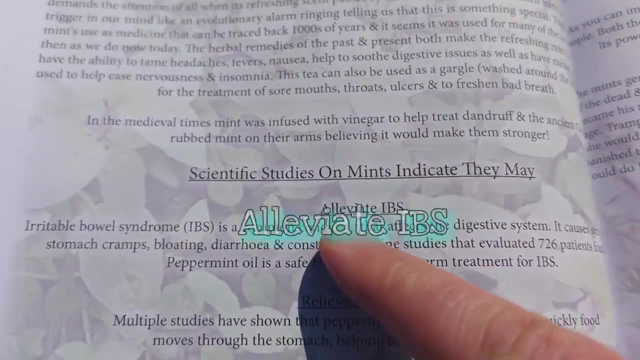 led science to dive into the world of the mint in the modern world today, and they found the mint had many medicinal properties and they all reinforced the traditional ones that our ancestors understood so well. When science dived into the world of mint, they found mint can help alleviate symptoms of IBS. 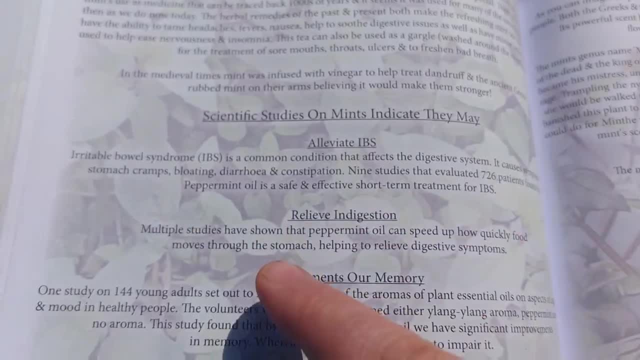 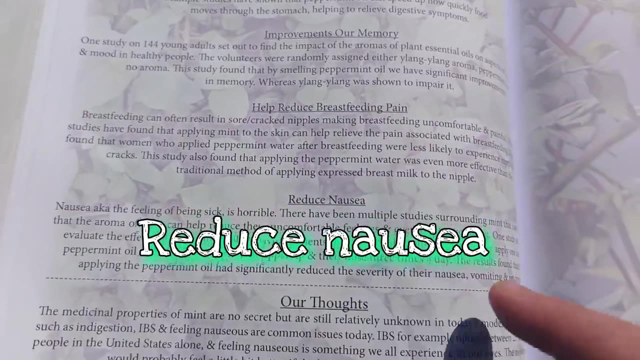 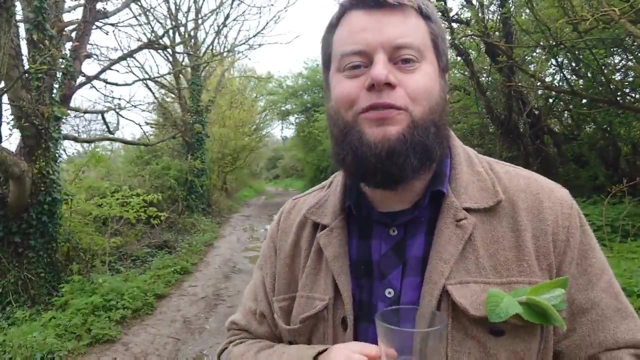 relieve symptoms of indigestion, improve our memory, help reduce breastfeeding pain and, of course, reduce the feeling of nausea. Isn't it fascinating how, when science dives into the traditional uses of plants, trees and fungi, that knowledge that's been passed down through time, that more times than not it's proven? 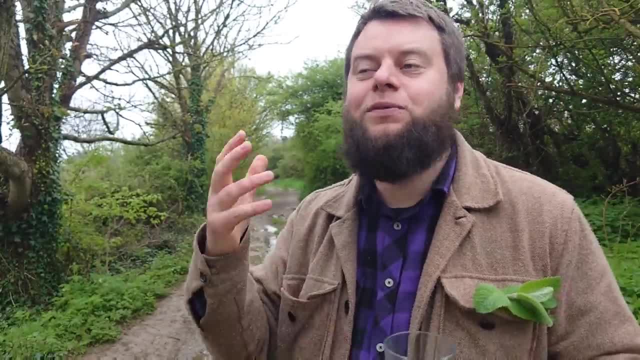 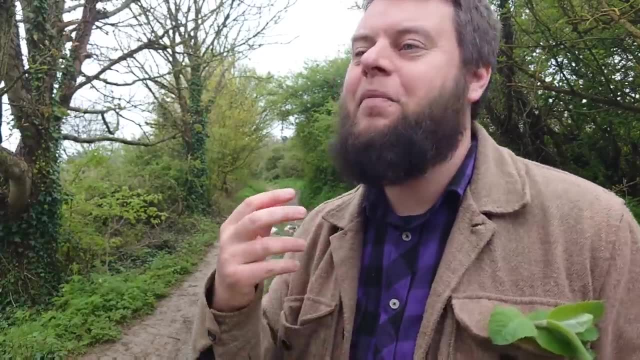 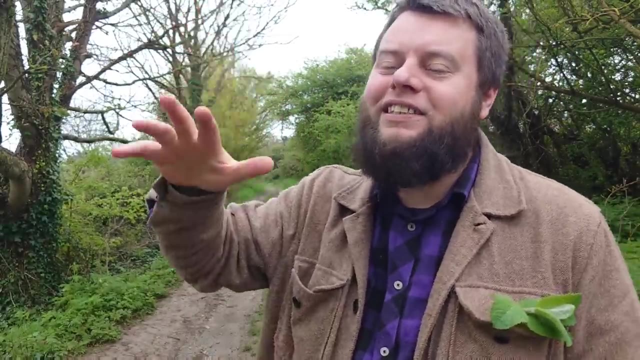 correct by science today. The mint can help us feel less nauseous when we're unwell and soothe our headaches. I also believe that the mint has a powerful ability to help bring balance to our minds. You see, certain plants, like lemon balm, can bring our minds down. 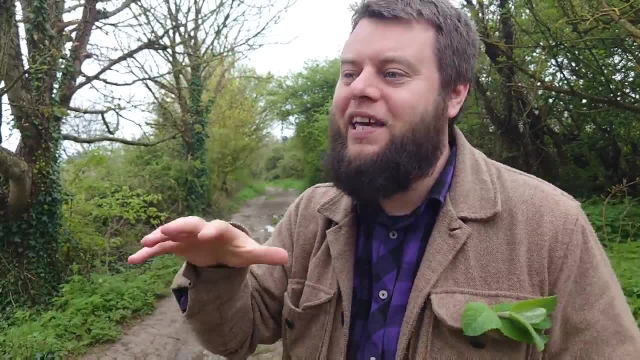 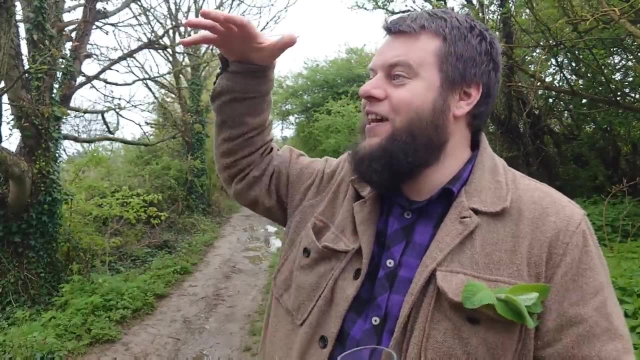 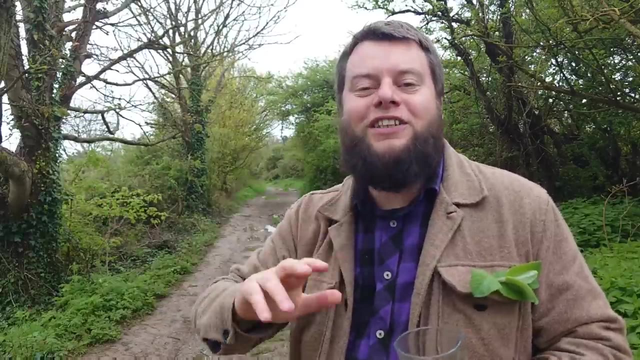 lower our consciousness to a place of calm and peace so we can reduce our anxiety and rest, Whereas other plants, such as mint, have the ability to elevate our consciousness and refresh us, bring us to a place of good vigour and help us wash away that lethargic mood. 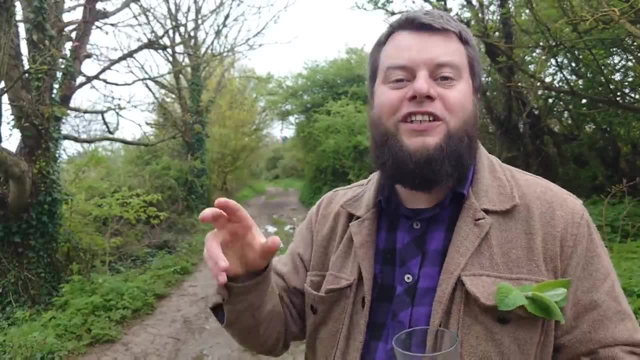 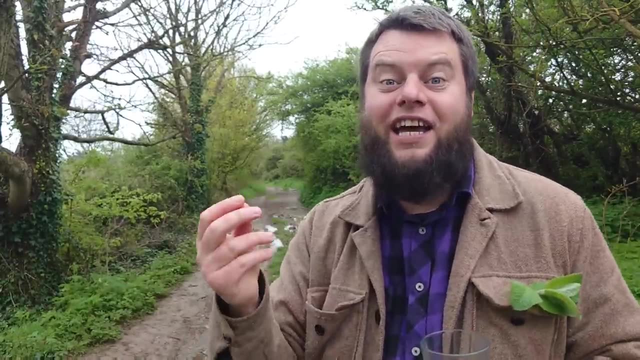 The next time you're in the world of mint, don't forget to subscribe to our channel, like this video and turn on your notifications so you don't miss any of our videos. Next time you're out or you feel low or lethargic and you just need an uplift, bring some mint into your life through a herbal tea or a wild and free snack, and you'll be surprised at just how much these plants can change our moods and how we feel. 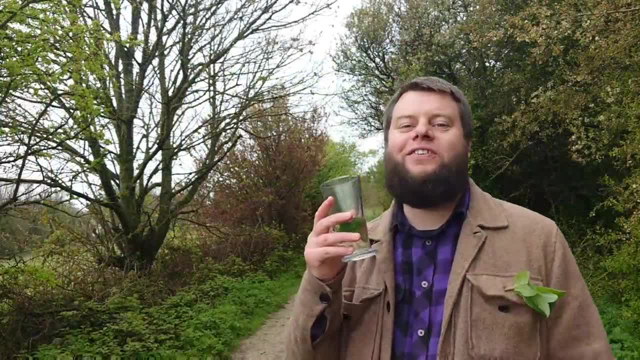 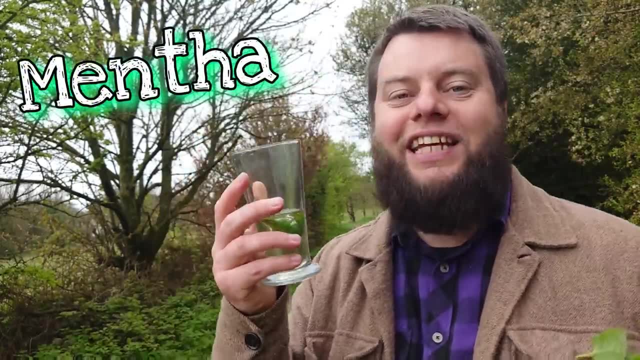 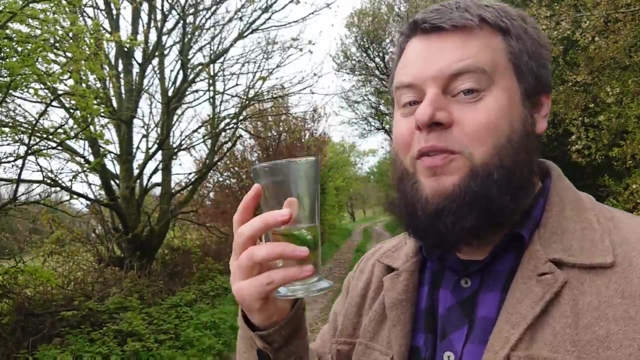 And we also know that mint's been loved by people for thousands and thousands of years, because even its Latin name, mentha, descends from ancient Latin, all the way back to ancient Greece. You see, there was a legend once of someone called Hades, and Hades was the lord of the dead and the underworld. He was pretty much the devil, and the story tells that there was this beautiful young nymph named Minthe, and Hades took a shine to this beautiful young nymph and made her his mistress. But unfortunately for Minthe, this was a terrible thing because Hades was married and it didn't take long for his wife, Persephone, to discover the love affair. And in a jealous rage she transformed Minthe into the first ever mint plant, so she would be crushed and walked upon forever. This broke Hades' heart and he couldn't undo the powerful curse. All he could do was cast another spell to give the mint plant an extra sweet, beautiful smell. 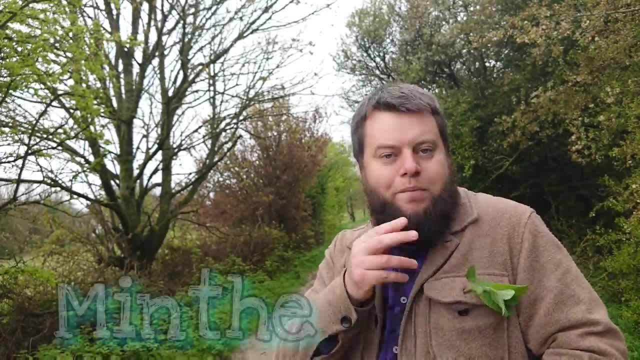 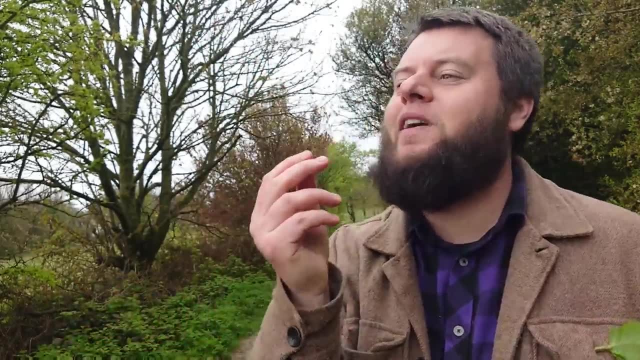 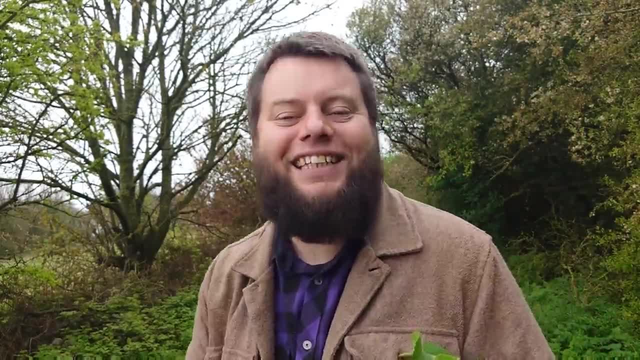 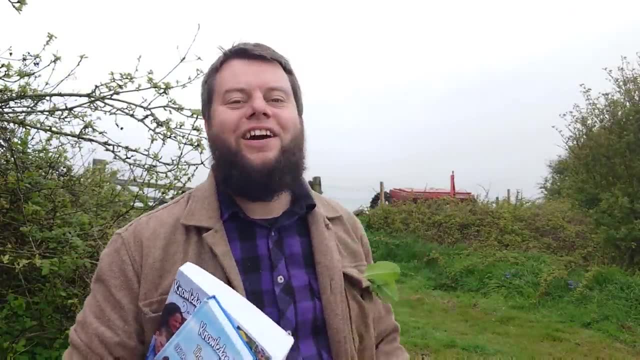 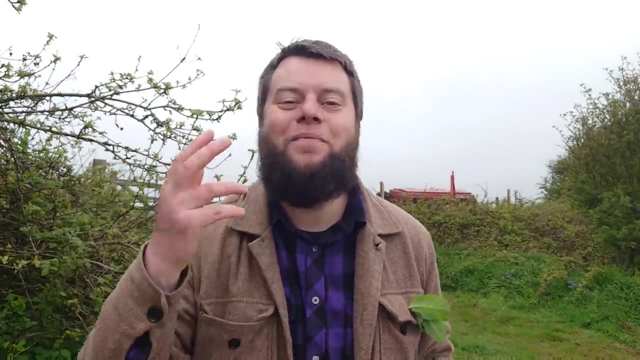 of the beautiful mint. so there we have it, people: the magical world of mint, a plant that can be found growing across the world, a plant that provides us with free food and medicine, a plant that transports our minds to a better place, and a plant that allows us to experience the sweetness. 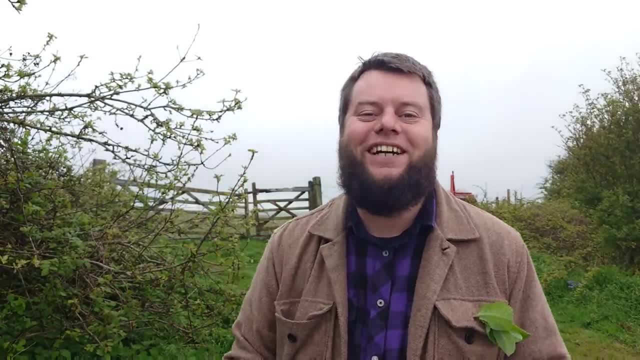 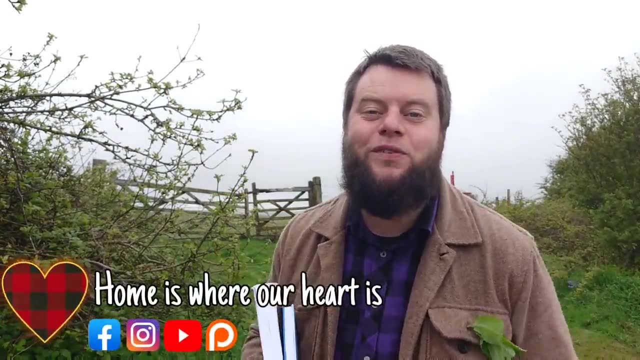 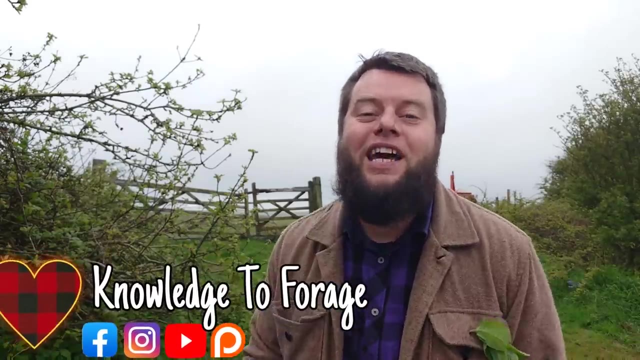 and freshness of magic from thousands of years ago. as always, people, it's been a pleasure. don't forget to do all the modern world things such as like this video, comment, subscribe, ring the bell, share it far and wide so we can share the magic of mint with everyone. and if you want to own all, 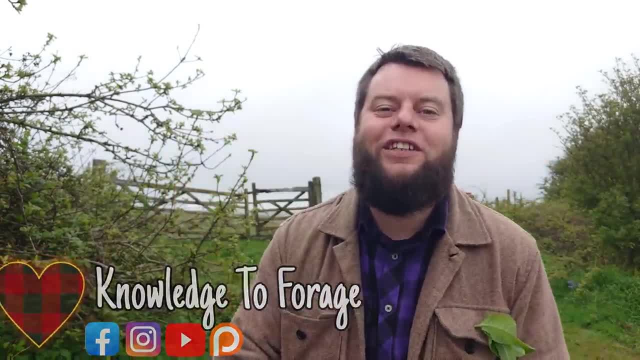 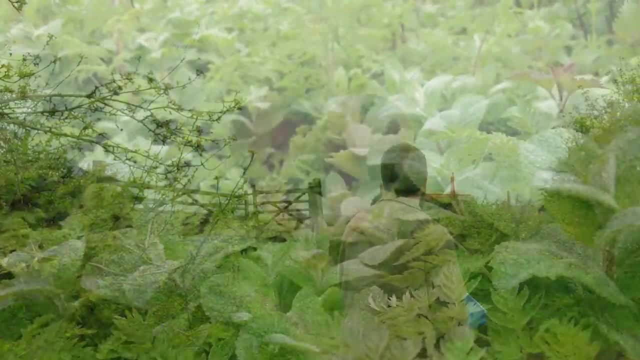 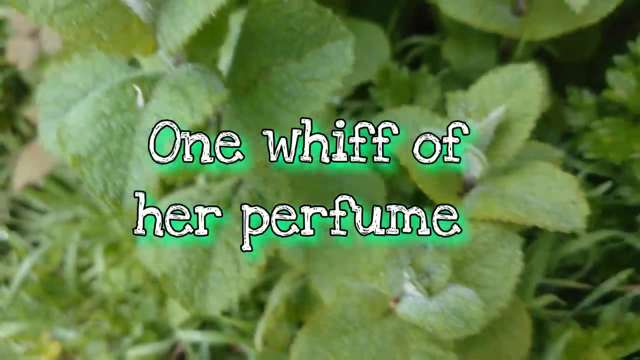 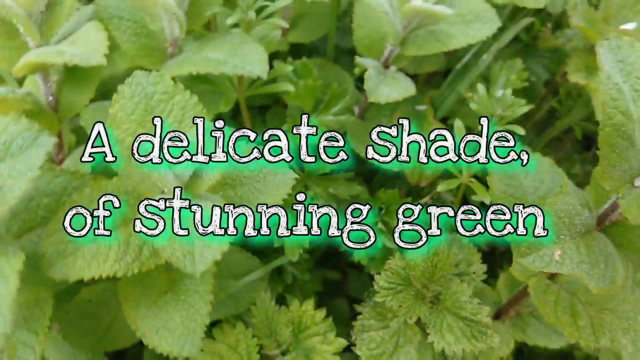 this knowledge in a big book, then check out our books. knowledge to forage, but most importantly of all, take care of yourselves and i'll see you all next time. peace, the marvelous mint with her beautiful, refreshing scent. one whiff of her perfume frees us from the grip of nauseous torment. minty, fresh and a delicate shade of stunning green.